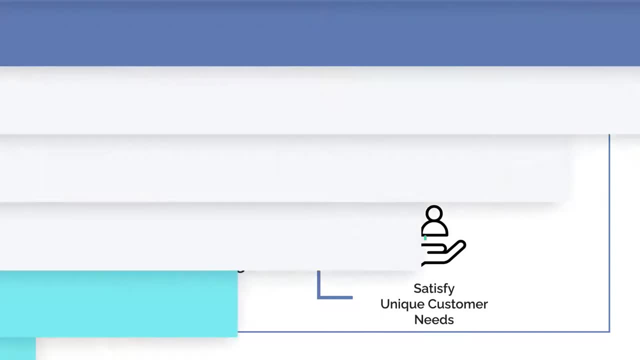 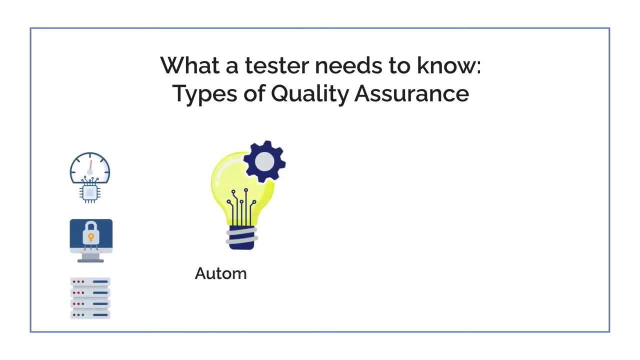 customer needs, provided you know which method to use and when. Automation testing. Certain software with multiple builds require repetitive testing with diverse datasets, which may increase chances of human error. Automation testing accelerates the process of functional as well as API testing to improve the test coverage, Reduce efforts, avail accurate results and, in turn, deliver quality product. 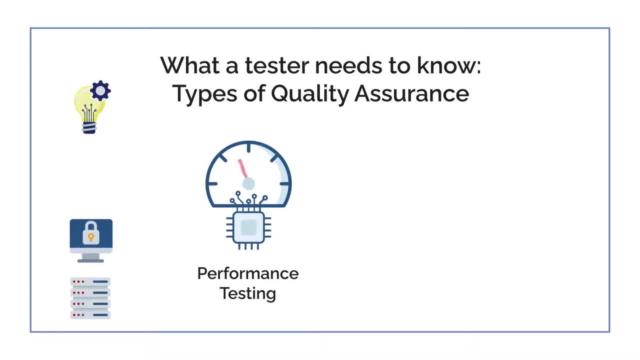 on time to the end user. Performance testing: Complex software often suffers from issues such as low speed, inconsistency across platforms and poor usability. Performance testing allows testers to determine how the system performs in terms of responsiveness under varying loads and equips stakeholders with information on scale. Performance testing allows testers to determine how the system performs in terms of responsiveness under varying loads and equips stakeholders with information on scale. Transforming software. 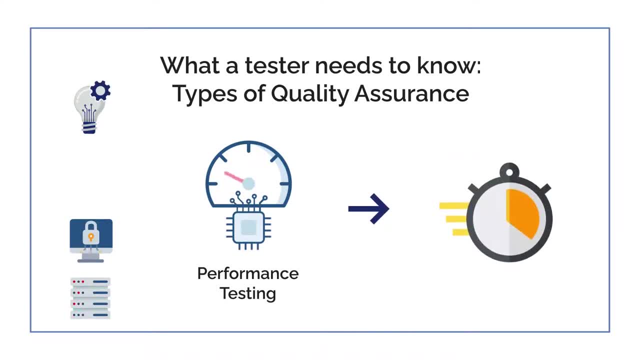 on stability, scalability and speed. Security testing- Vulnerable software can be easily exploited and, in some cases, even cease to function. Security testing enables testers to denude the flaws in a system and ensure that it is protected from potential intruders. to keep 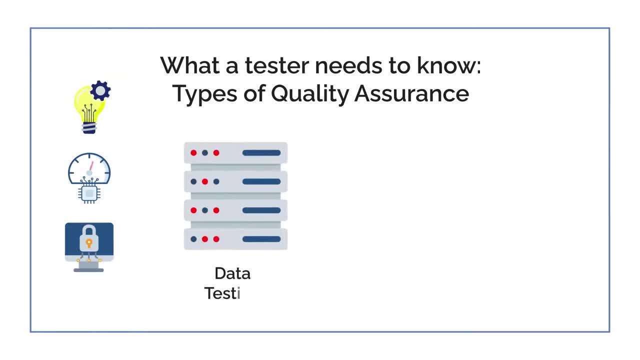 the data safe and maintain desired functionality. Data testing: Business decisions are made after a thorough analysis of data, making it imminent to conduct data validation. With security testing. testers perform end-to-end data validation for various applications to confirm whether correct data is presented in the application, thus ensuring confidentiality, integrity. 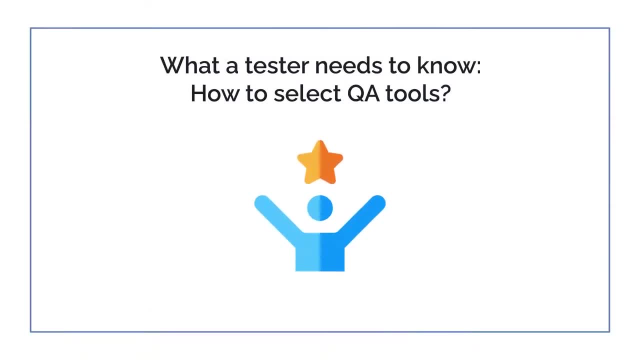 and availability. In order to achieve consistent results with minimal efforts, the tools used in QA should be selected after ensuring that they are standardized, compatible, cost-effective, efficient, scalable, robust. Following are the essential languages and tools that every tester must have. 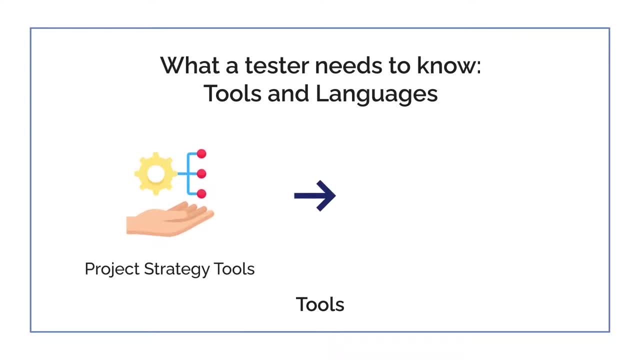 in their arsenal: Tools, Project Strategy Tools, Agile, Scrum, Kanban Boards, Project or Sprint Planning Tools, JIRA, Pivotal Tracker, Active Collab Communication Tools, Slack, Microsoft Teams, Yammer Document Repository Tool, SharePoint Test Repository and Defect Management Tool. 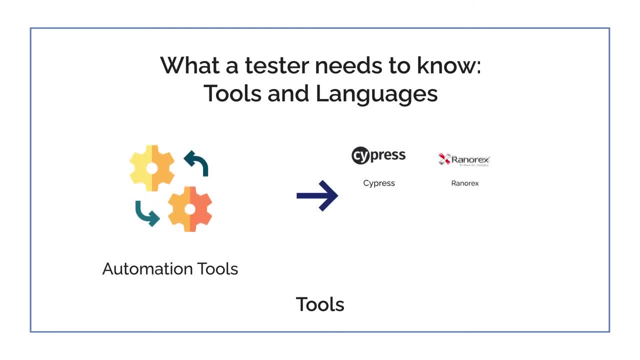 JIRA Automation Tools, Cypress, RANRX, Karate, APM, Selenium, Cucumber, CICD Tools, Jenkins, Git, Bitbucket, Cloud Build, Amplify, Azure Pipeline Test Management Tools, Cucumber Studio, X-Ray, Zephyr, Azure DevOps.